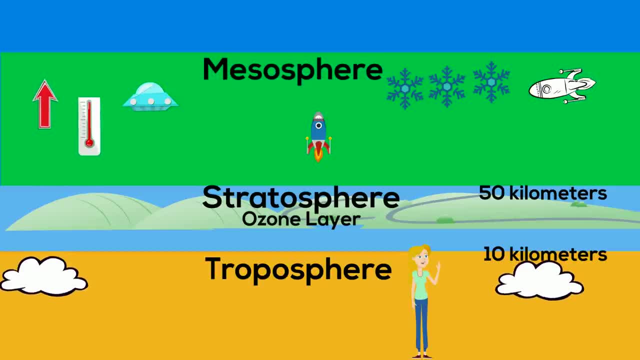 Stratosphere. The Mesosphere gets colder as you go up. In fact, it is the coldest layer and can have temperatures as low as negative 90 degrees Celsius. The Mesosphere protects the earth from space jump because the ice crystals burn up. the space jump as it moves. 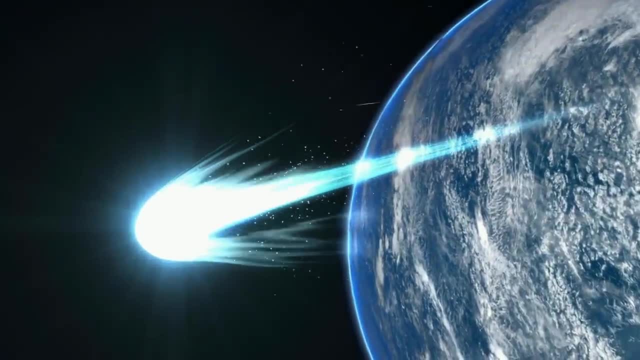 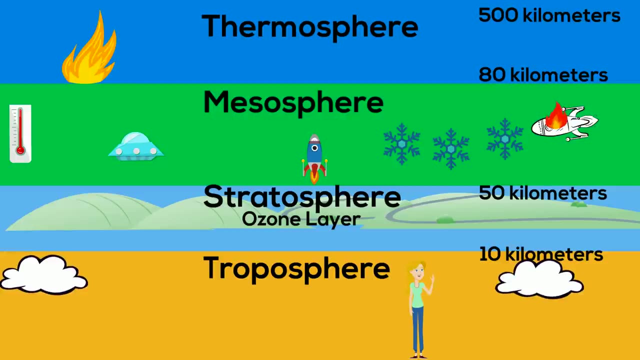 through it and extends to about 80 kilometers high. And finally you have the Thermosphere. This is very hot, In fact it is the hottest layer, and you can have temperatures between 500 and 1500 degrees Celsius at the very top. 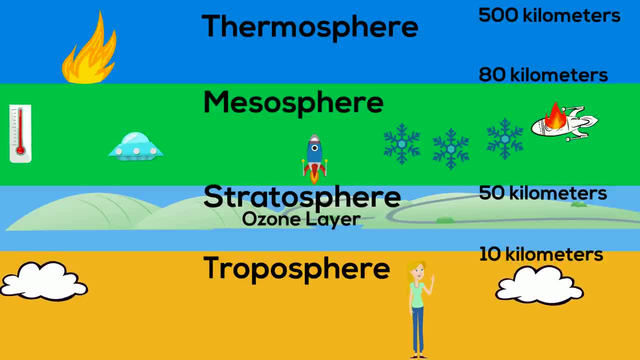 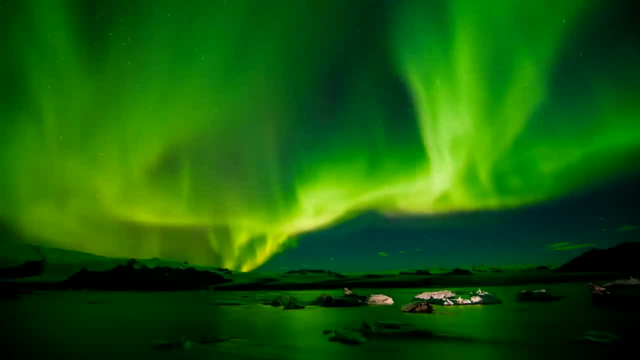 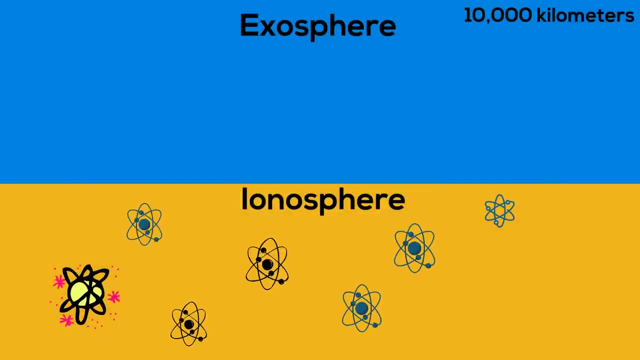 Two additional layers of our atmosphere is the ionosphere, full of electrically charged atoms and is the home of Northern and Southern Lights and also reflects back radio waves. The exosphere is the outermost layer of our atmosphere and stretches almost 10,000 kilometers. 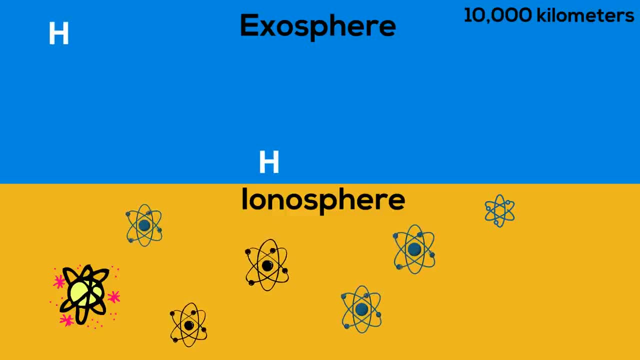 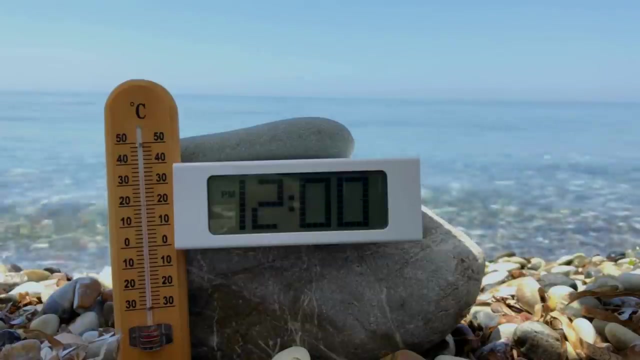 into space. It is composed of helium and several heavier molecules, including nitrogen, oxygen and carbon dioxide, but they are spread far apart. It is also home to the satellite- Two satellites. Each layer is classified according to temperature As you gain elevation in the troposphere. the temperature actually drops. The temperature range is from around 15 degrees Celsius to negative 45 to 50 degrees Celsius at the top. The temperature of the stratosphere actually gets warmer with elevation and ranges from minus 45 to 50 degrees Celsius at the bottom. 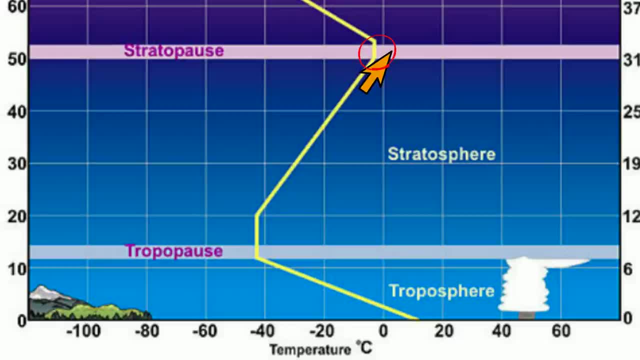 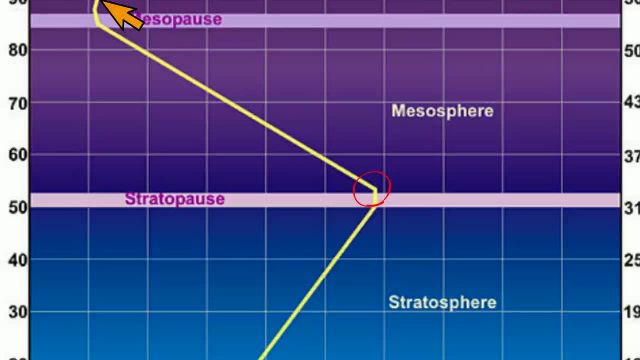 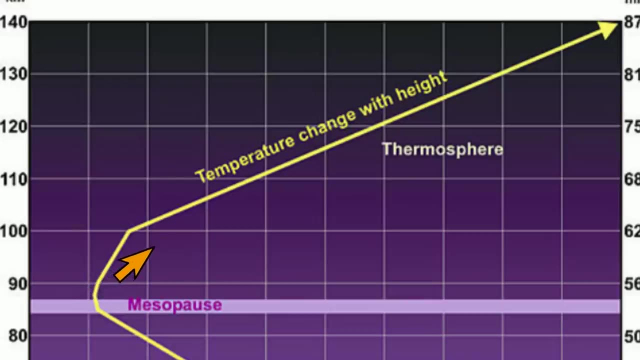 to zero degrees Celsius at the top. The mesosphere is similar to the troposphere and the temperature decreases with elevation. The temperature ranges from zero degrees Celsius to negative 90 degrees Celsius at the top And finally, the thermosphere actually gets warmer with elevation The temperature. 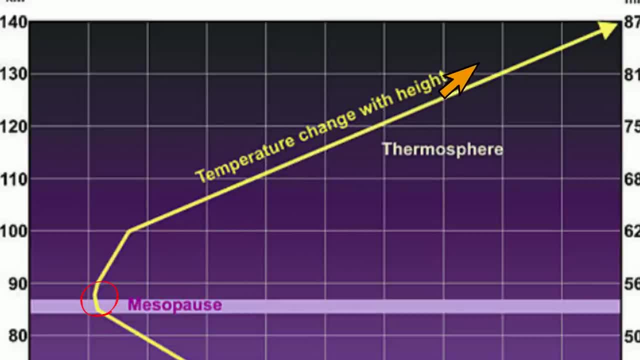 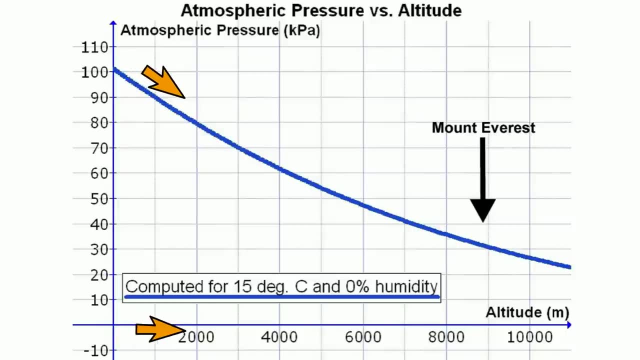 ranges from negative 90 degrees at the bottom to over 1500 degrees at the very, very top. Also, as you move from the troposphere to thermosphere, in other words get higher in elevation, the atmospheric pressure decreases. So as you go. 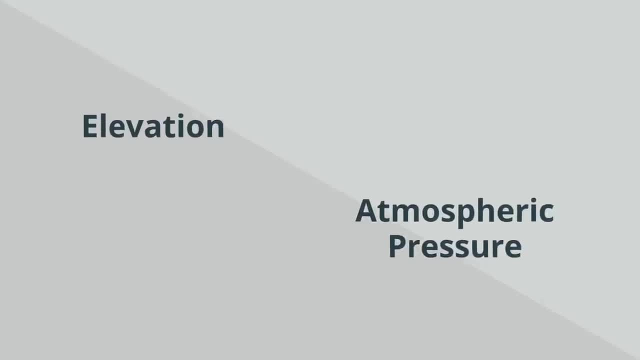 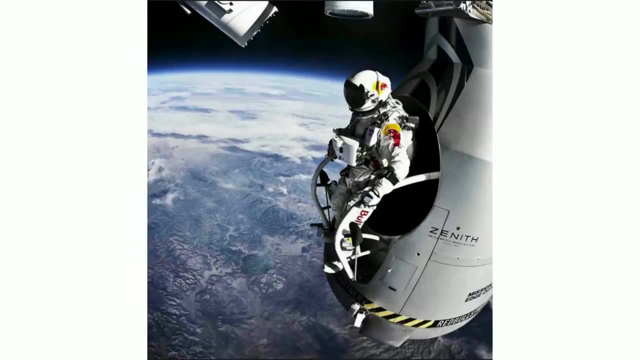 up in elevation, the atmospheric pressure decreases, And as you go down in elevation, the atmospheric pressure increases. In fact, in 2002, Felix Baumgartner completed a free fall parachute jump from the stratosphere And during this jump he reached speeds of over 800 miles an. 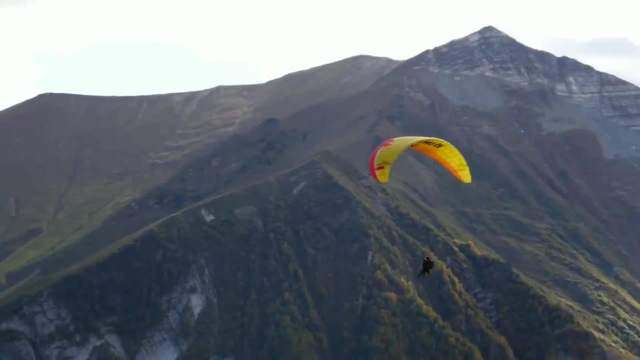 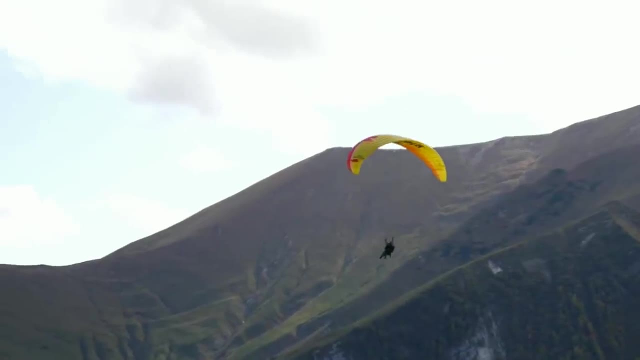 hour and even broke the sound barrier. He was able to reach these speeds because of the atmosphere was so thin that there was very little friction to slow him down. If you'd like to know more about the atmospheric layers, this playlist will help, And, as always, 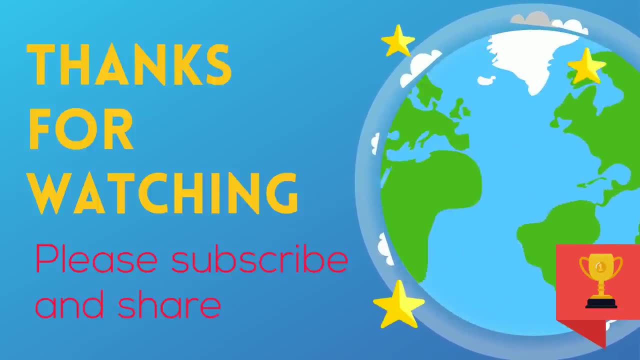 thanks for watching, And MooMooMath uploads a new math and science video every day. Please subscribe and share.